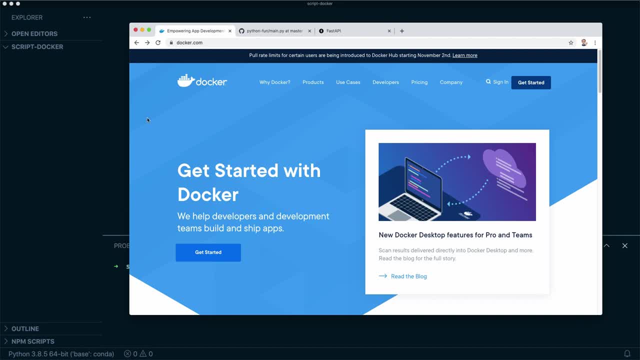 Hey guys, today I want to show you how you can use Docker for your Python application. I show you all the essential stuff to get started, And then we take a look at two different projects and how we can dockerize them. The first is a simple script that needs additional dependencies. 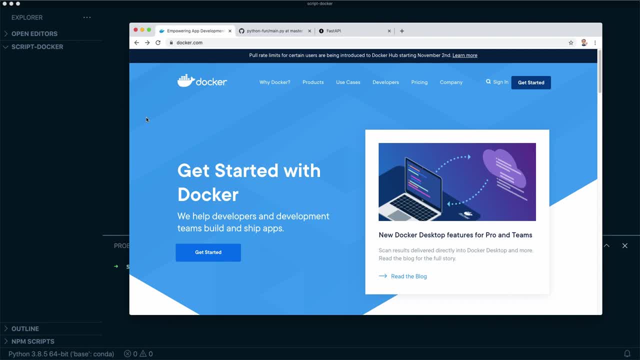 And the second project is a web application with fast API. This second example also shows how to dockerize a virtual environment, So this example is one of the most common use cases for Docker, And if you follow me here, then you should be able to apply this for all your own projects. 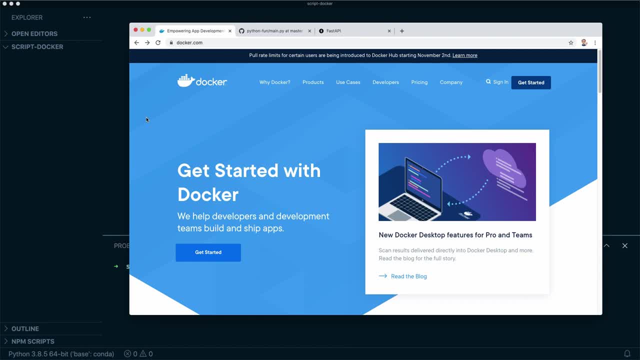 Alright. so first of all, what is Docker? In simple words, Docker is a tool that lets you put your application into a container. These containers allow you to package up the application with all of the parts it needs, So all the libraries and all other dependencies, and then we can deploy it as one package. 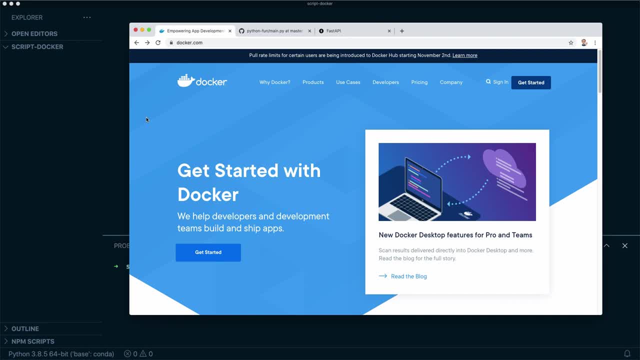 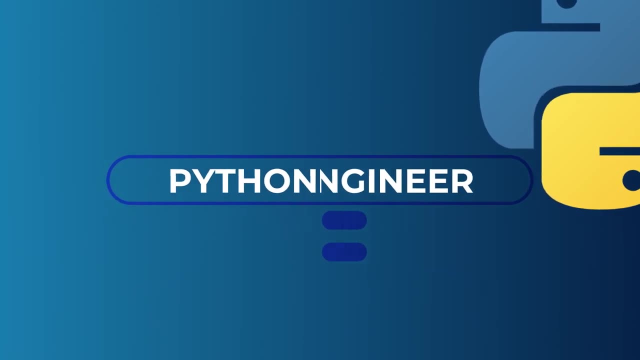 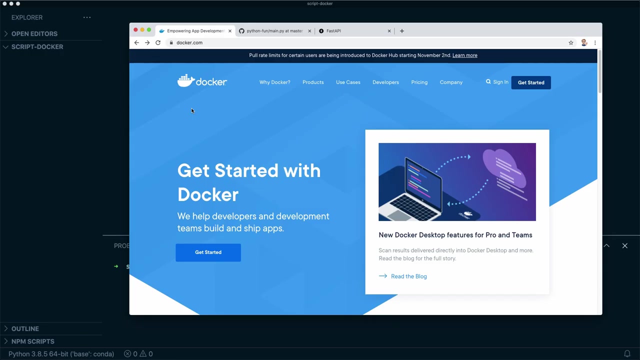 So if another one is using this, then he or she doesn't have to worry about installing all the correct dependencies first, So we can start using this right away. Okay, so now let's start dockerizing our Python applications. First of all, we have to install Docker, of course, So for this you can go to the official. 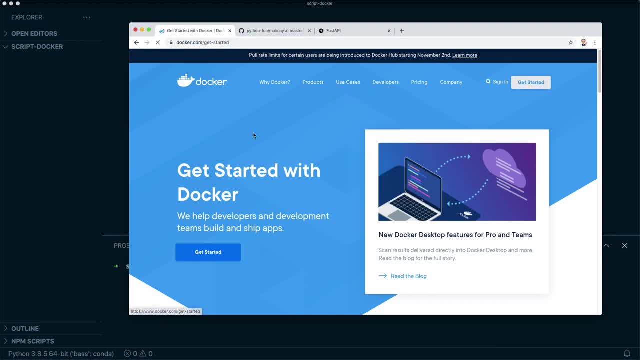 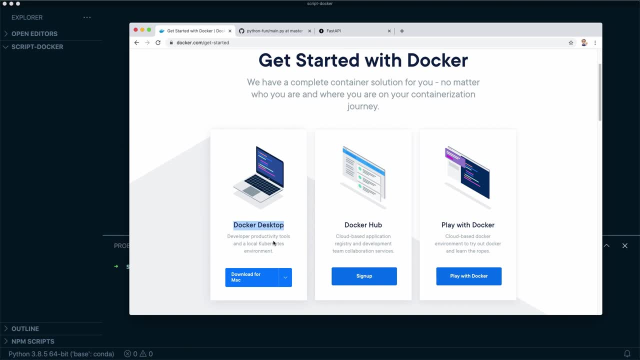 homepage: dockercom, Dockercom, Dockercom, Dockercom, Dockercom, Dockercom. Click on Get Started, And then I recommend to download and install Docker desktop. So this gives you both the command line interface and also a useful desktop application. 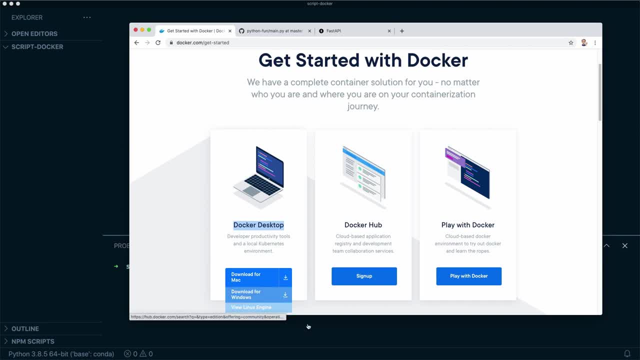 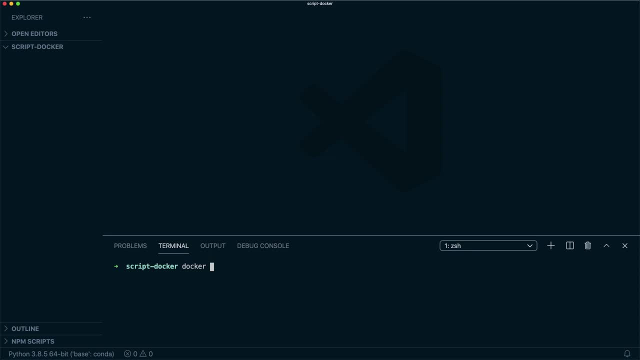 So choose your operating system and download this and follow the installation guides. And once you have installed this, you can verify this in your terminal by typing in Docker minus V. This should tell you the current Docker versions. So yeah, here we can see that I already have this on my machine. 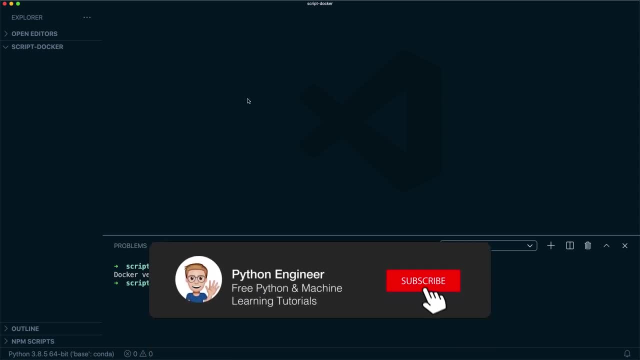 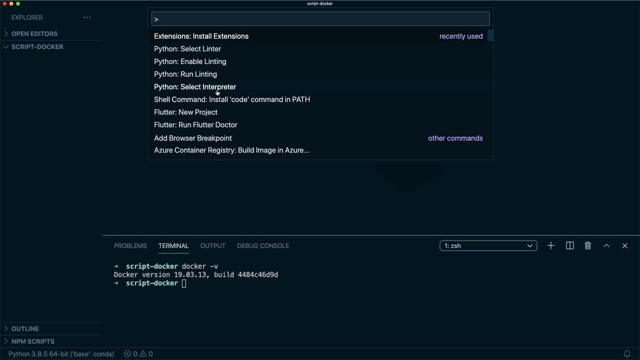 Alright, so this is working, And here I'm using Visual Studio Code as my editor, And if you're using the same, then I also recommend to install the Docker extension, So you can go to the command palette, type in install extensions and then here search for. 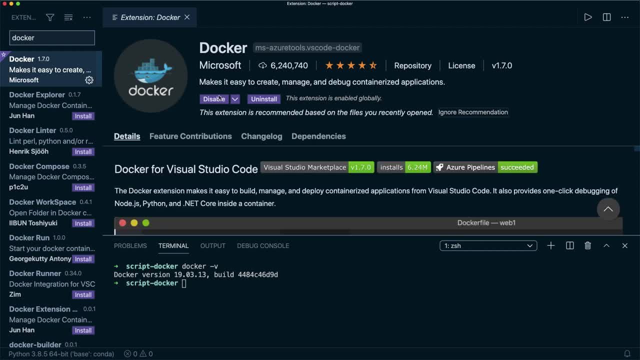 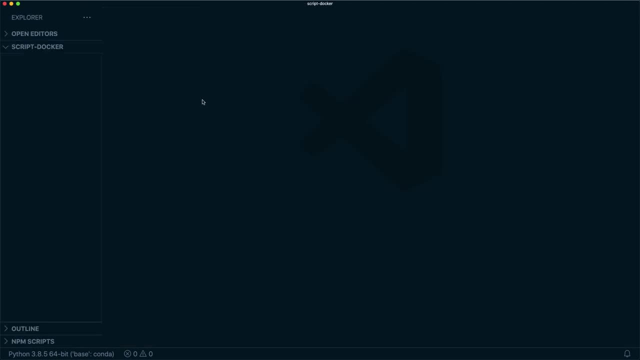 Docker and use the official Docker extension from Microsoft. So I already installed this And this is what we're going to install this on gives you nice features, for example, for debugging or for auto completion. So go ahead and do this, And now we can start docker raising, our first Python script. So for the first, 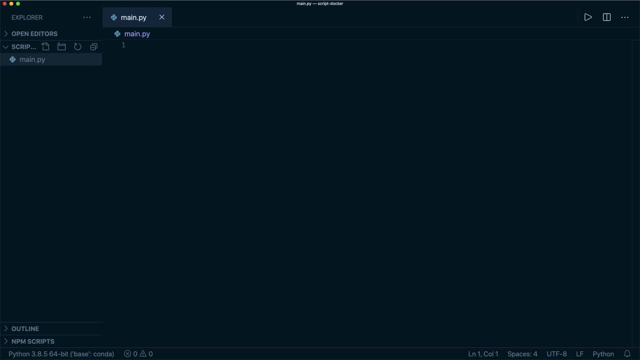 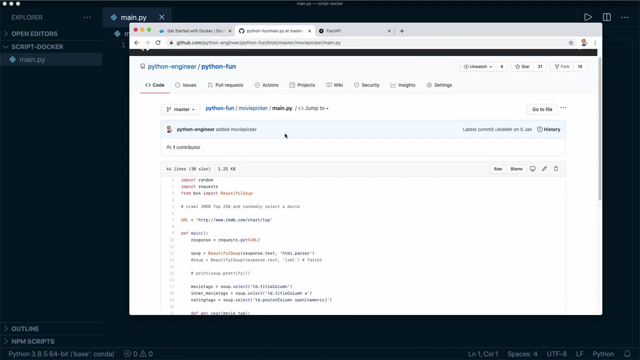 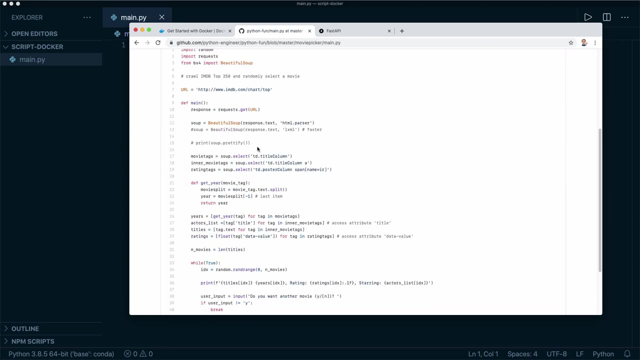 example, I want to have a single Python script, main dot pi- And for this example I'm going to use the code from another tutorial that I already have here on my channel. So this is the IMDb movie scraping tutorial, where I scraped the IMDb charts and then randomly 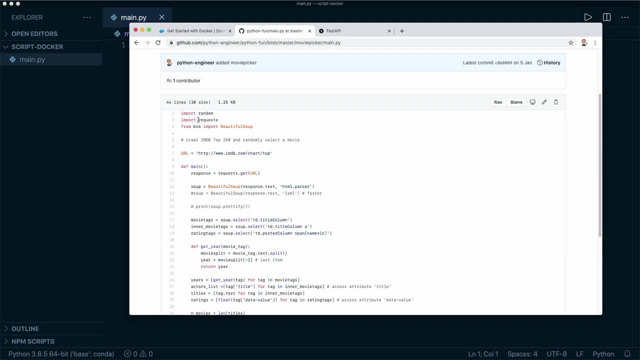 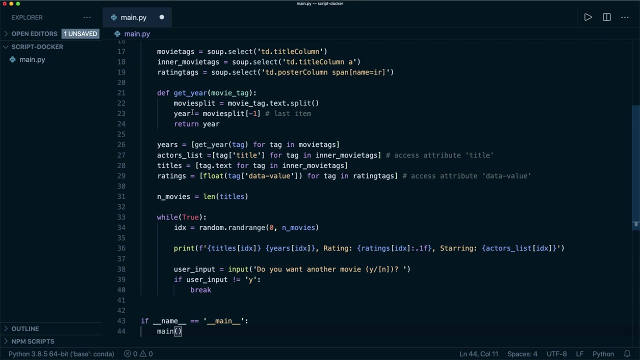 suggest a movie. So this uses the requests library and beautiful soup, And if you're interested in that, then go ahead and check that tutorial out as well. So I will put the link in the description. So now I simply copy and paste this And here I'm dealing with. 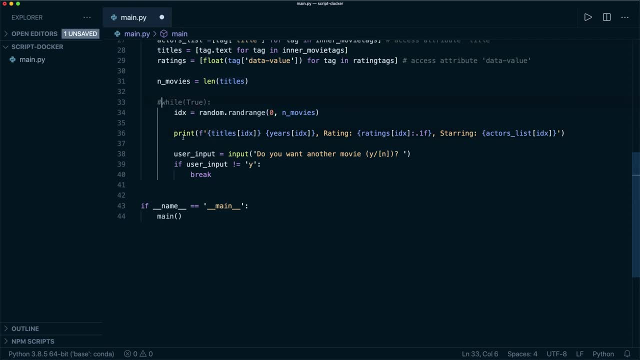 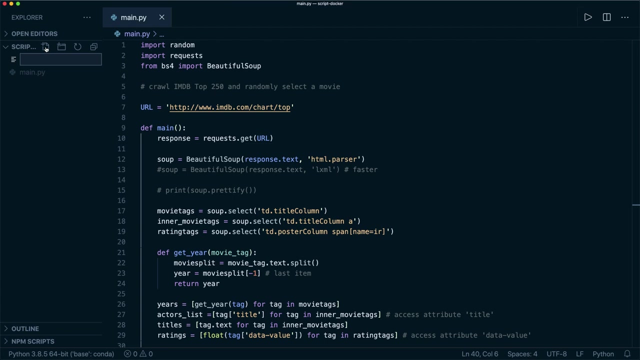 a user input as well. So for now, I comment this out, but I will show you how we can use this in a second as well. So let's comment this out. So now we can start stocker rising this, and the first thing we need is a Docker file. 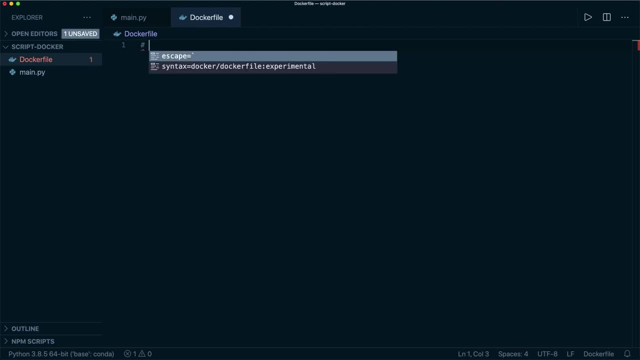 So we have to differentiate between three different things. The first one is the Docker file, Then we have the Docker image And then we have a Docker container. So a Docker file is a blueprint for building images. A image is a template for running containers. 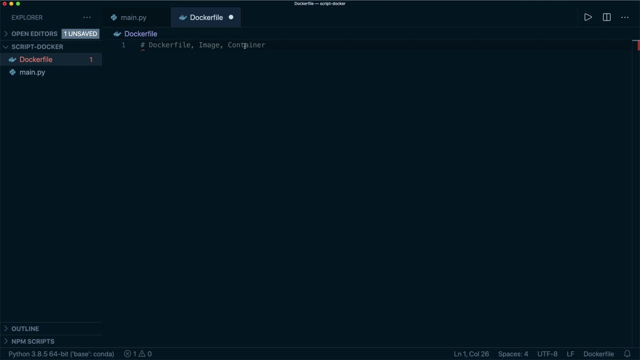 And the container is then the actual running process, where we have our package project. So the first thing we have to do is to define our Docker file- And, by the way, we can use comments in here like this- And the first thing we have to do is specify a base image. 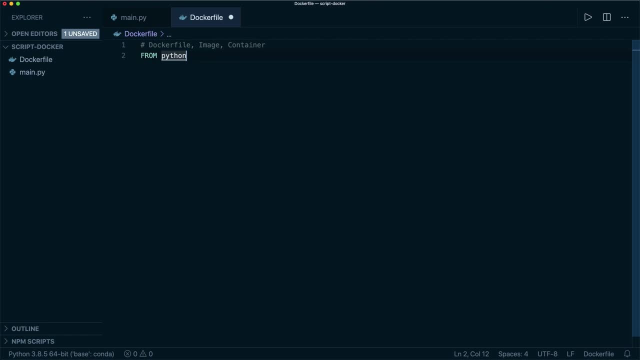 So here we can say from, and then use Python, and then colon, and we can specify the version of 3.8.. So this is pulling this image from Docker Hub, which already has Python installed. So we have all the things we need to have Python in our container. And now the next. 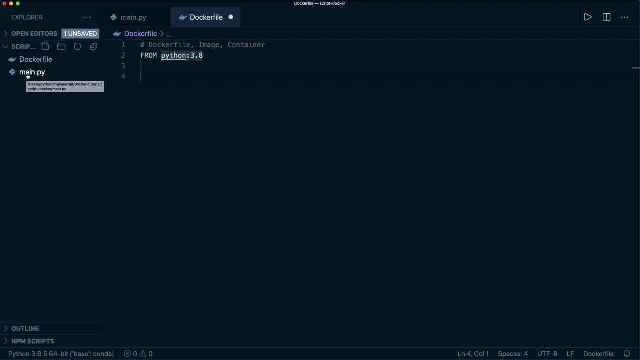 thing we want to do. we want to add this mainpy file into our container. So we do this by saying at, and then the source is mainpy And the destination is just a dot, So in the current directory in our container. Now that we have that, we have to install the dependencies. 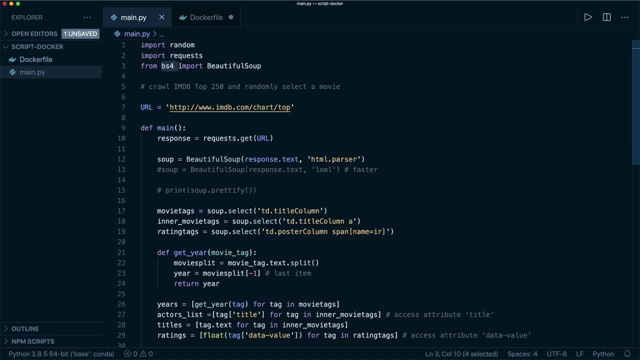 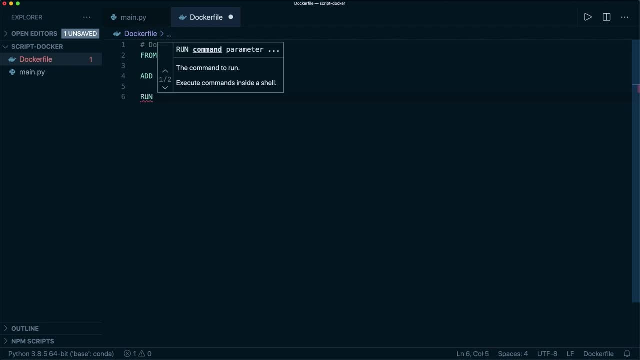 So, as I said, we are using requests And beautiful soup, So we have to install them with pip And we can do this by saying run and then simply the command pip, install requests and also beautiful soup, And I guess the pip package is called beautiful soup for. So now that we have that and then the last 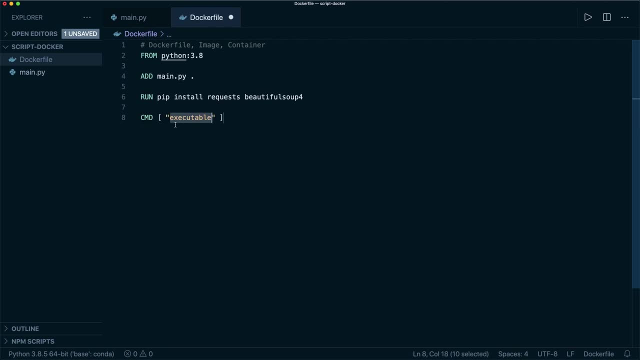 thing we have to do is specify the entry command When we start our container, And here we want to say python, And then, as second parameter, here we say colon, slash and then mainpi. So this is simply a running Python mainpi. 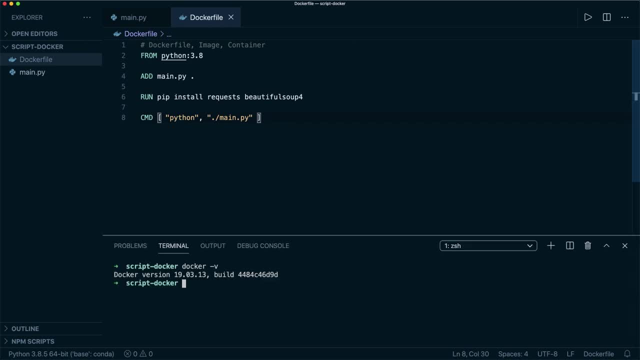 in our container terminal. So now we have all four, our Docker file, And now we have to create our Docker image. So we do this with the commands Docker, build and our docarus, And then this is the return in container. So we have the next thing we want to do here. is to add this in our container, And now we have all the stories from our Docker file. And also we have to add our PAC server, And now we can add our VM wenig to this file. And now we have to create our Docker image. So we do this with the command Docker build. 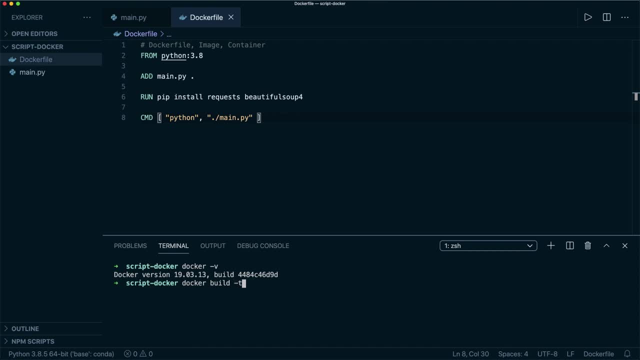 default minus t for tag and then the name of the image. So I call this Python, I am the P and hit Enter, And I also have to specify the location. So here I simply use a dot again And now it's building the image And, as you can see, this is executing these steps in. 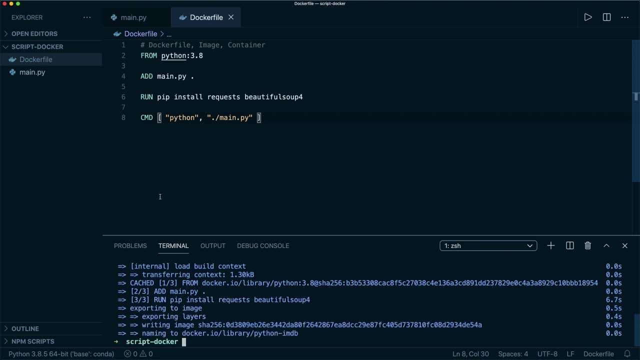 this order. So the order is important. So it's pulling the Python image, then it's adding main dot pi, then it's installing the modules and then we are done. And then when we start our container then it's running this file. And then we start our container by saying: 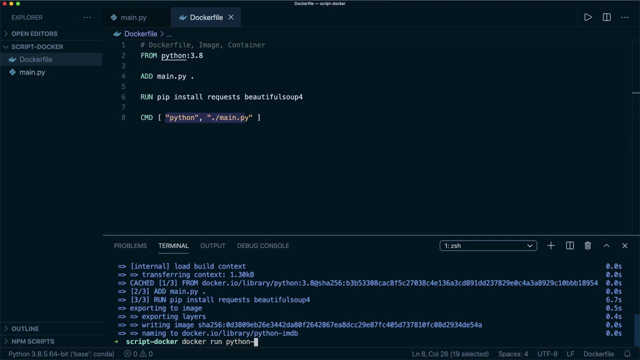 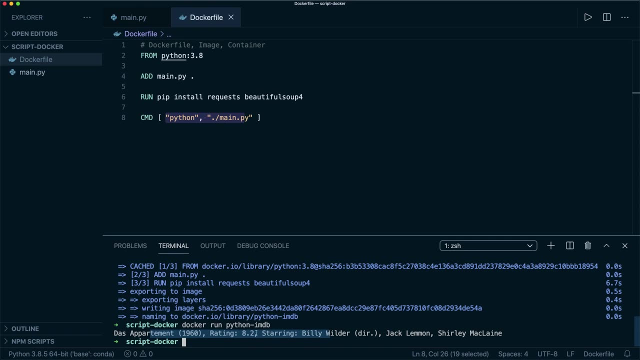 Docker run, and then the name of the image- Python, imdb- And then we see that our container is starting And the script is running and we get a random movie suggestion And then our container comes to the end, So it's shutting down again. So now we can try this again, And then we should. 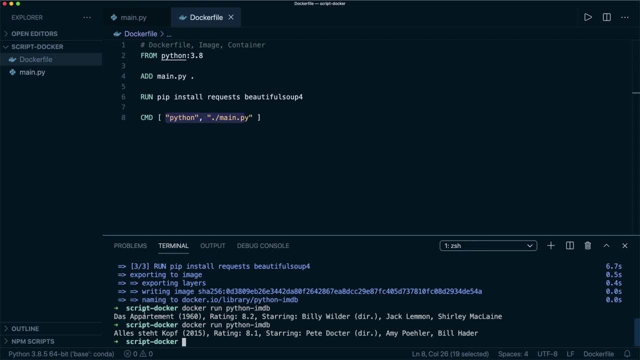 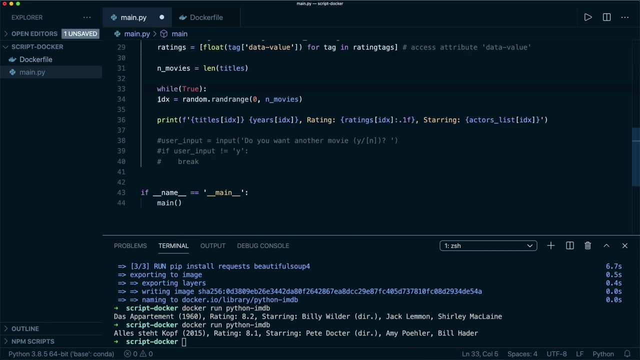 get another random suggestion. Alright, so this is working. And now, as I said here, I commented out this part where we use the user input. So now let me put that in the description again. So now we have the complete script and save this, and then we have to build. 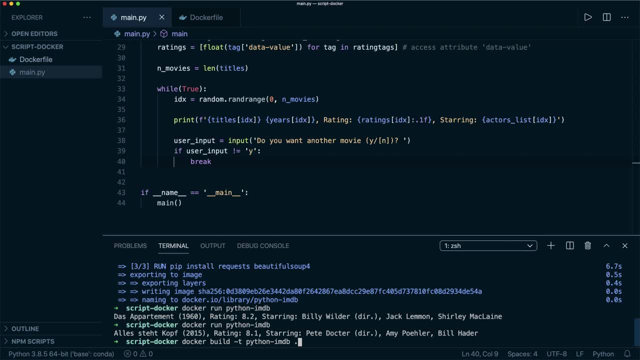 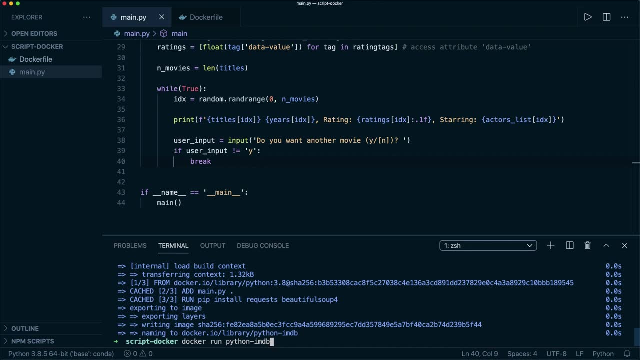 our Docker image again. So again we run this command. And now if we start our container with this Docker run command like this, then it will crash. So yeah, so we see we get this EOF error, And this is because, for if we use a user input, then we have to use additional arguments for the Docker run command. 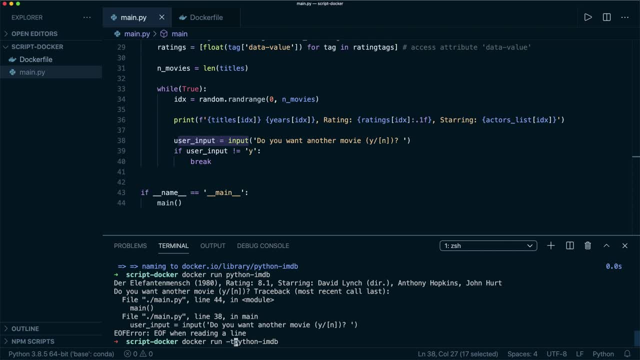 So we have to say: Docker run minus t and minus i. So the I stands for interactive mode and the T will give us a pseudo terminal and where we can type in the user input. So now, if we run it like this, then this should work again. 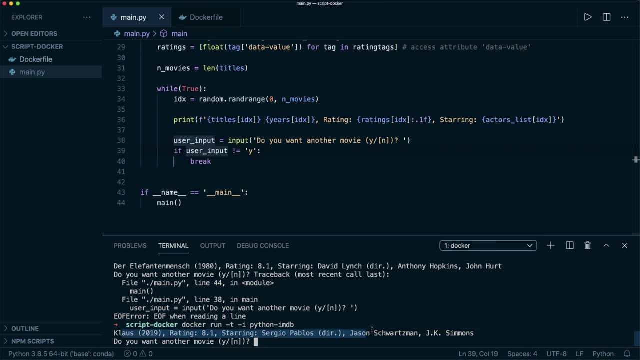 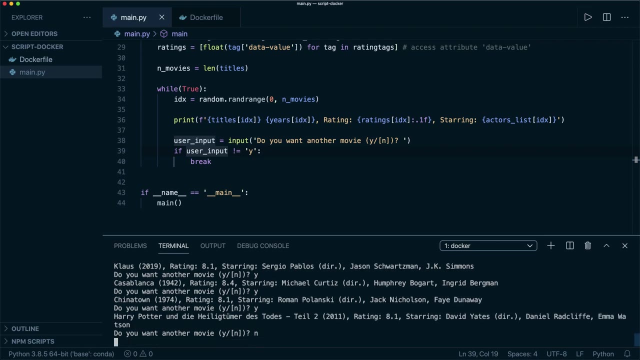 Okay, alright, so now this is working. So we get a movie suggestion And then it asks us if we want to see another movie. if I say yes, then this should give me another one, and yes and yes. so this is working. And then if I say no, then this should end this script and 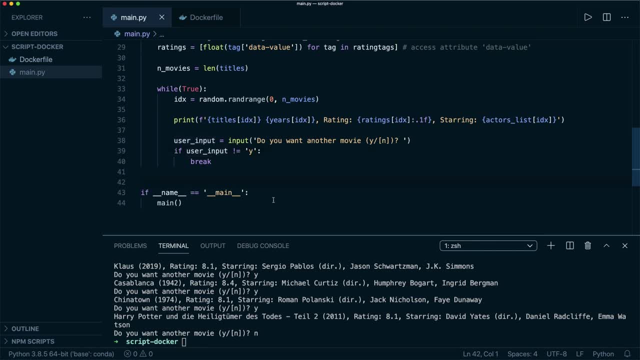 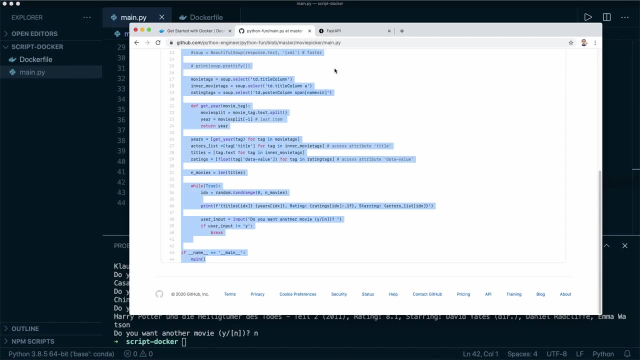 also ends the container. Alright, so this is working. And this is the first example. Now let's have a look at a more advanced tutorial. So for the second example, we're going to start off with the use of this label. So for: 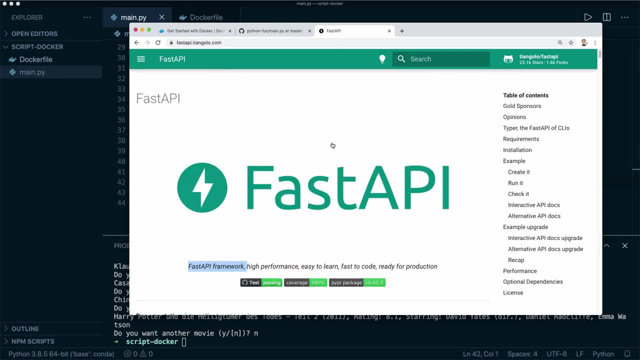 this example, we're gonna take a look at a look at a more advanced tutorial. So, for this example, I want to create a web application with the fast API framework, But this basically works the same for every other web framework that you use. So we start by creating a virtual. 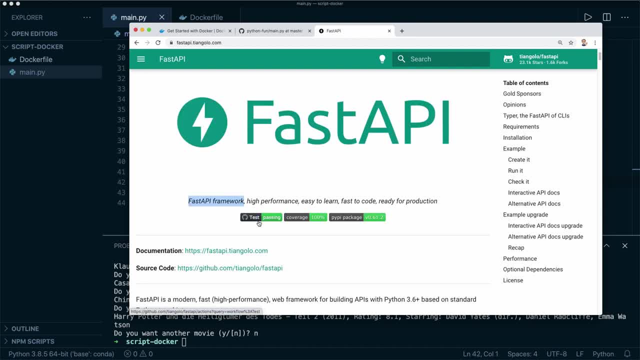 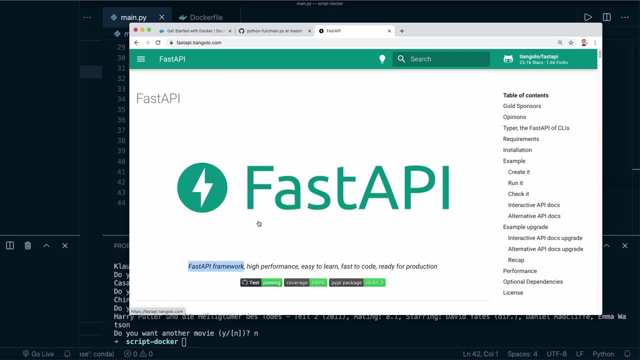 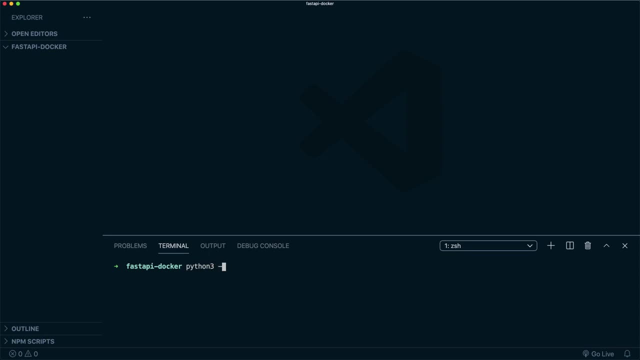 environment, then install the dependencies and then write our application and then dockerize it. So let's do that. Alright, so here I'm in a new empty directory And the first thing I want to do is create a virtual environment. So I do this by saying Python, three minus. 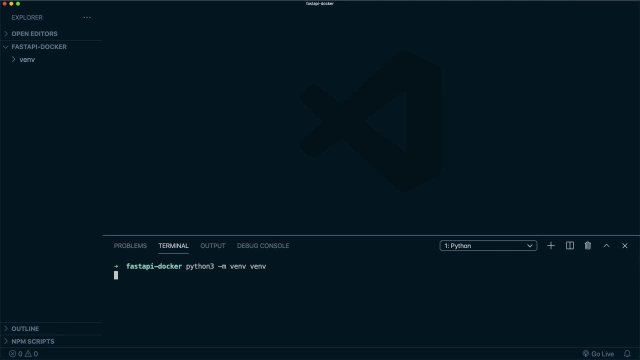 mv and v, and this command might be slightly different on Windows. And now we created it and then we have to activate it by saying dot v and slash bin, slash activate. And again, this command might be slightly different on Windows. And now we are inside this virtual. 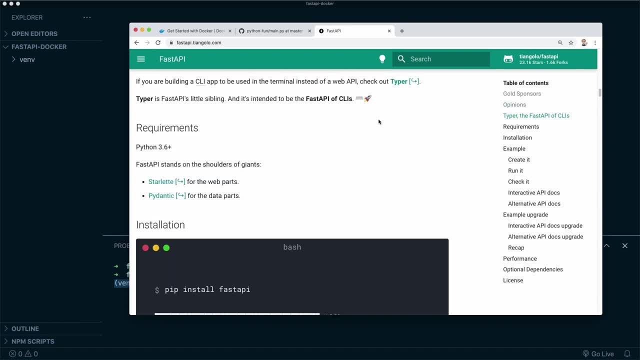 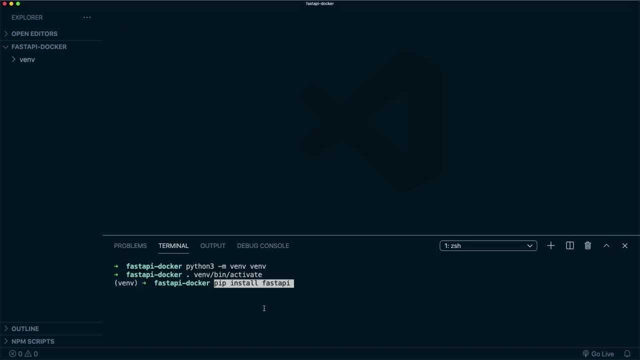 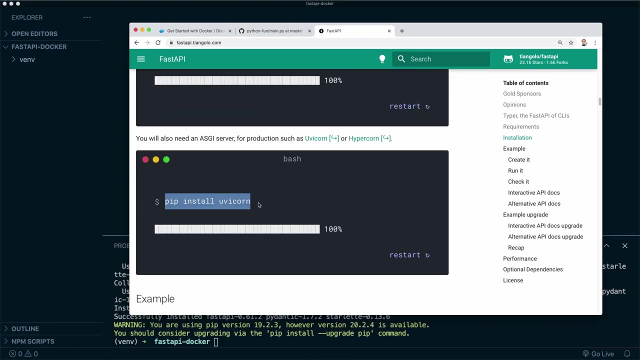 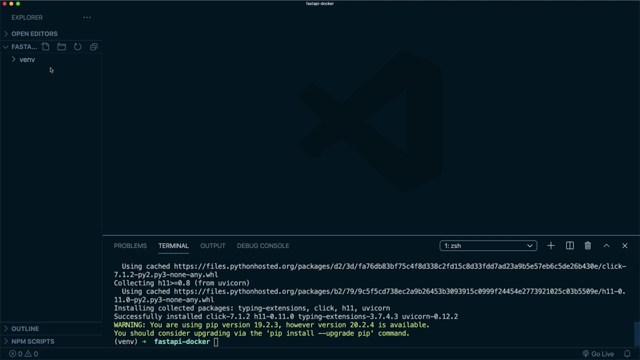 environment. So now we install the dependencies, in this case for fast API. So we say, pip, install fast API. And we also need a web server. So we say, pip, install UV corn and hit enter. So now we have that. And now let's create our app. So let's create another directory in here and then the file. 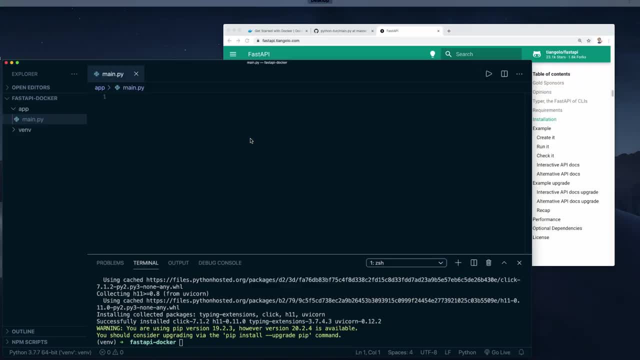 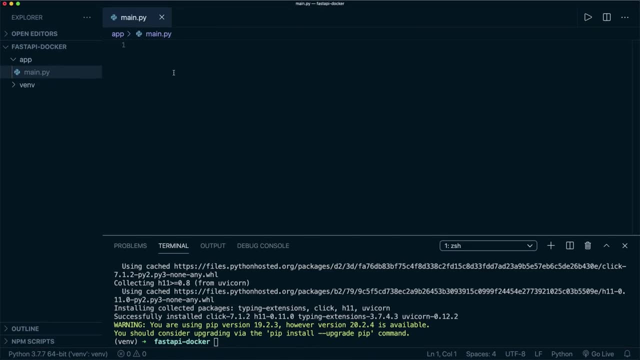 main dot pi in this directory. And now let's grab the example code from the website, So this one here and paste it in here. So this syntax is very similar to the last syntax. So we create an app and then we define our functions, where we define the routes And 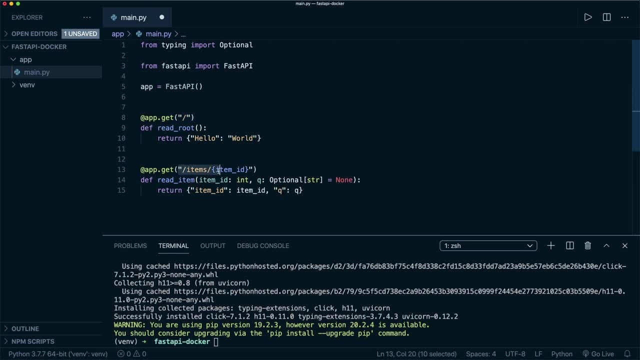 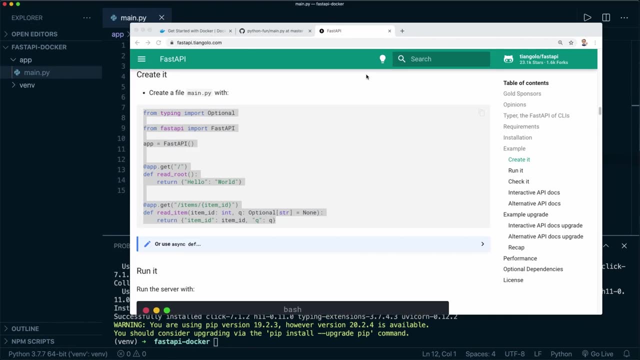 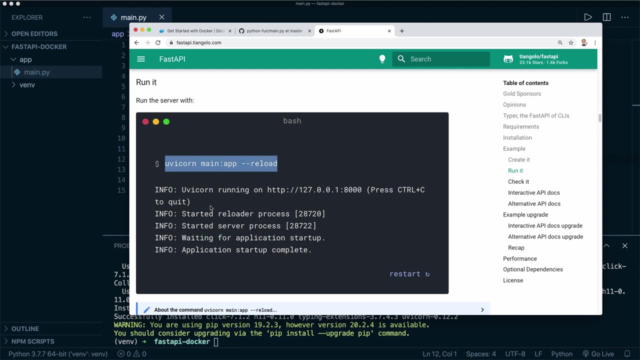 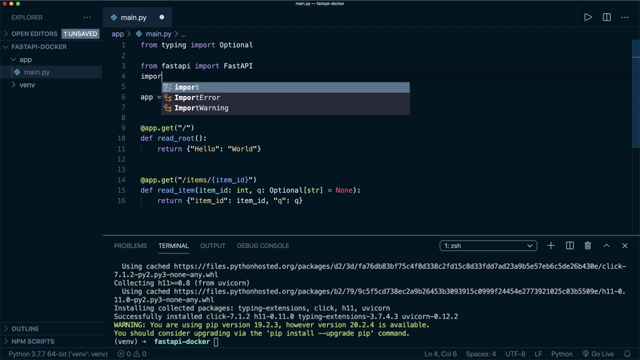 now they, we set the up and let the drill, ms t set, import the UV corn library, And then we say: if name equals, equals main, and then we say: UV corn dot run, and then we want to run our app. So this is, I think, the same or very similar. 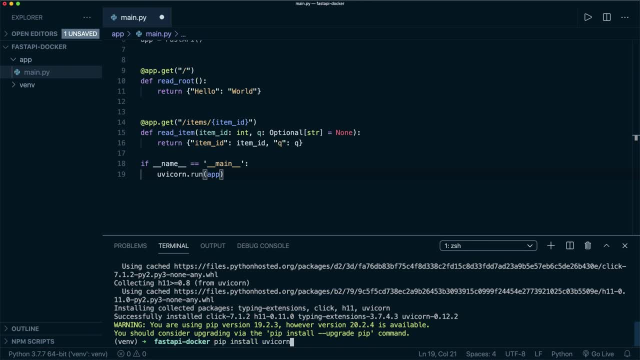 with flask. With flask you can also start it from the terminal. Or you can start it with flask dot run inside here, or app dot run- I guess it's with flask, So yeah, so let's do it like this. And then of course we have to run the script. So now we say: 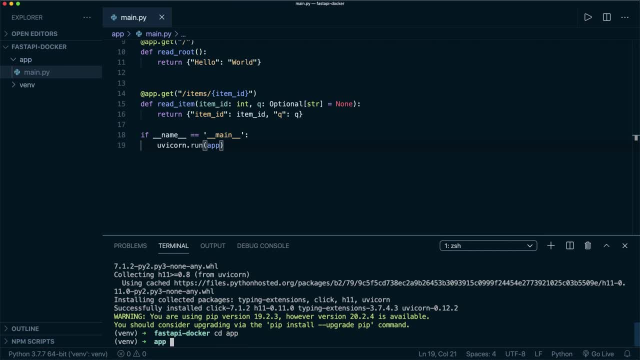 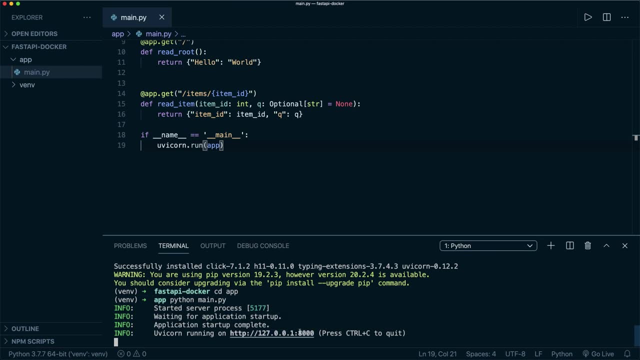 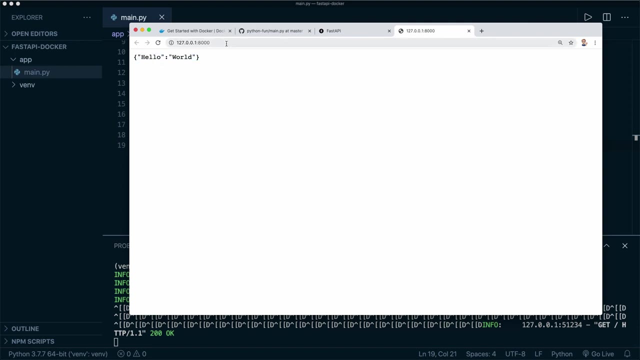 let's go into the app directory And then let's say Python, main, dot pi, And it says that our server is up and running. So we can go to localhost 8000.. And we see, we get the Hello world response. So this is working. And if we go to slash, 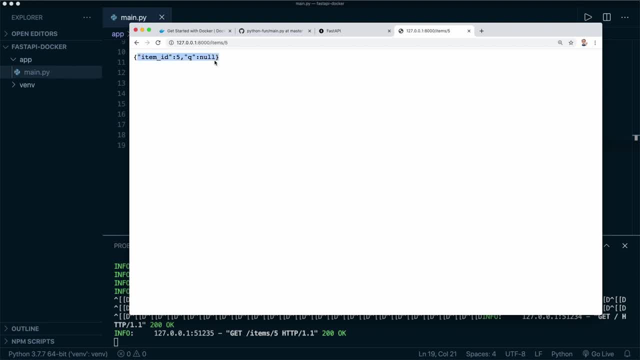 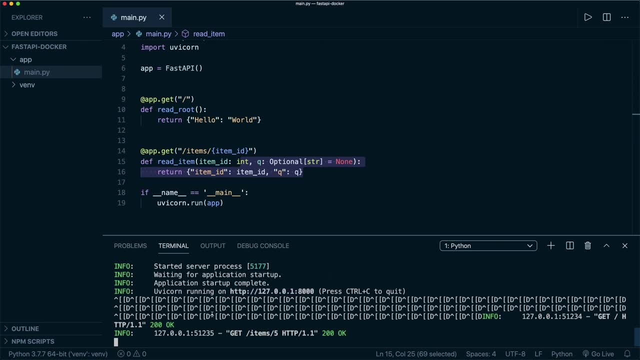 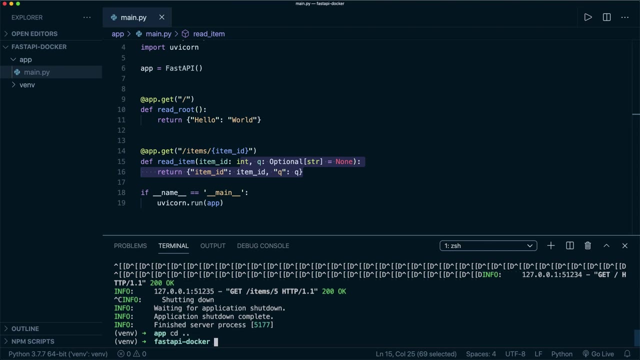 items, slash item ID. then we get the second response that we specified. So yeah, so this is working. So let's shut down the server again And let's go back to the root directory from this project, And let me clear this. So now we want to dockerize. 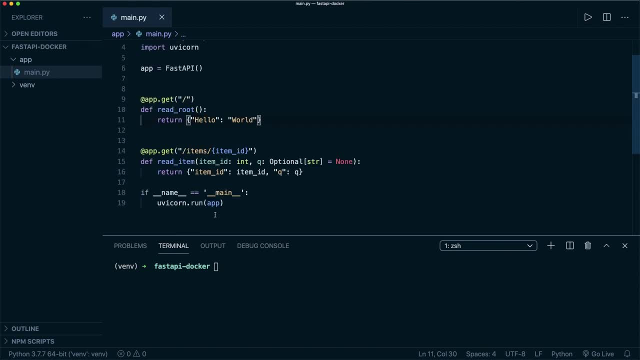 So the first thing we want to do is to save all the dependencies in a requirements txt file. So for this we say pip freeze and then the greater sign and then require man's dot txt. So this writes all the dependencies that we just installed into this file. So 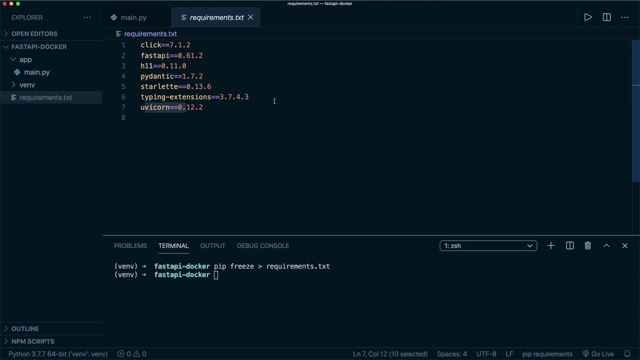 we see, we have fast API, we have unicorn and some other dependencies. So the next thing we want to do is, again, we want to create our Docker file, Docker file, And this should be in the root directory of our project. And here again, we start by specifying a base. 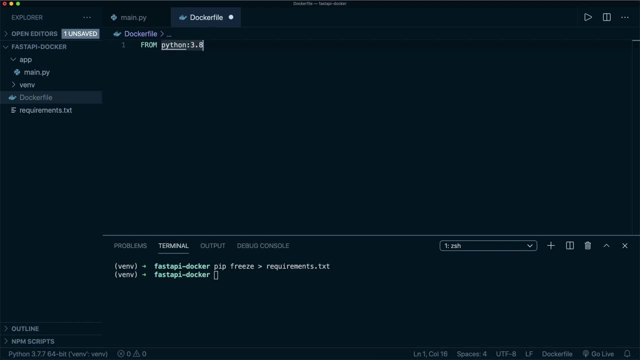 image. So here again we say Python and version 3.8.. And now I want to do something new, So I want to organize the folders in the container in a slightly better way. So I create a working directory with this command, And then let's. 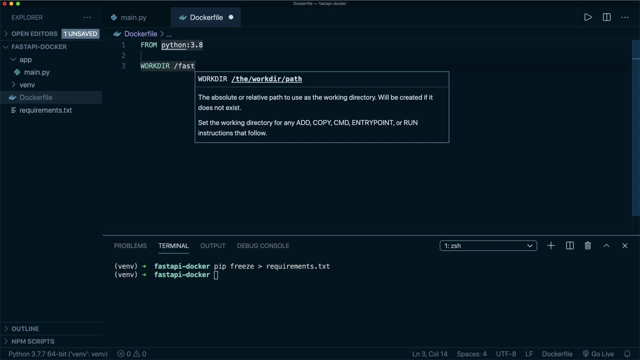 call this directory in this container, fast API dash app, And this will also automatically go into this directory. So now, this is our starting point, And now we want to copy the require man's dot txt into this working directory. So we simply have to say colon, then we have to install the dependencies. 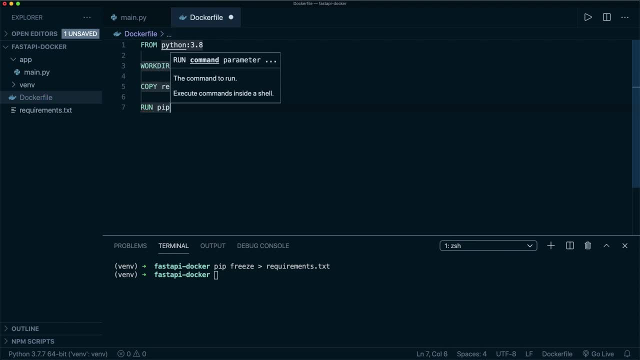 And we do this again with the run command And this time we say pip- install and then minus our request, And we do the same thing with this configuration. So we are going to copy this from the US directory. So what we do here in our use this is: we go to this directory and we're going to make a new one, And the next thing we want to do is to copy this whole app folder with the main dot pi file. So let's do this by saying copy. And we want to copy from dot slash app. So this is the folder here on our machine And then we specify the folder name inside. the container. So let's also call this app. So now we're going to do a backup property And while we're doing that, let's run thedateback, And then we do the same thing here. So now we're going to do like the build and save to the donwit command, And this time let's just go into our 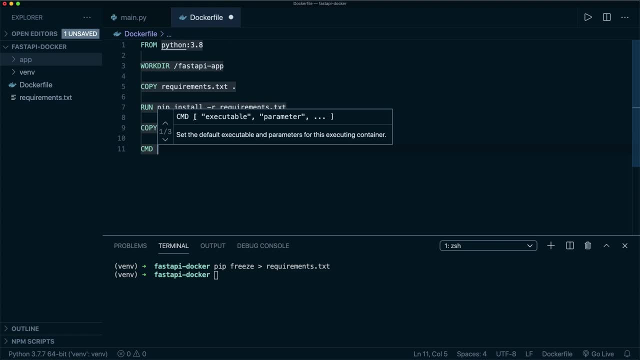 So now we have that, And now we also have to specify the entry point for our container. So again here we use the command Python And then we want to run the mainpy file. So this is in the dot slash app folder, and then slash mainpy. So now this is our Docker. 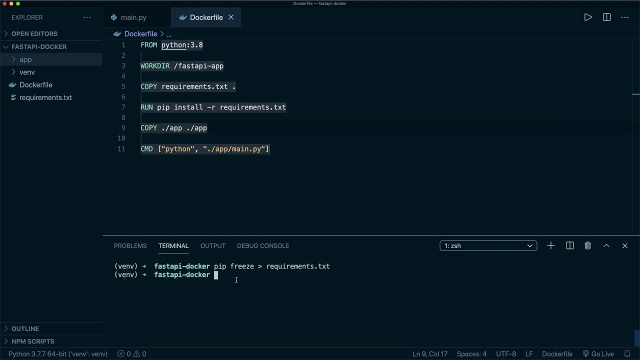 file. And then again we have to build our image. So we say Docker build minus T, And then let's call this Python minus fast API. And again I forgot the dot here. So again with the dot at the end for the current location. So now this is running and executing all those. 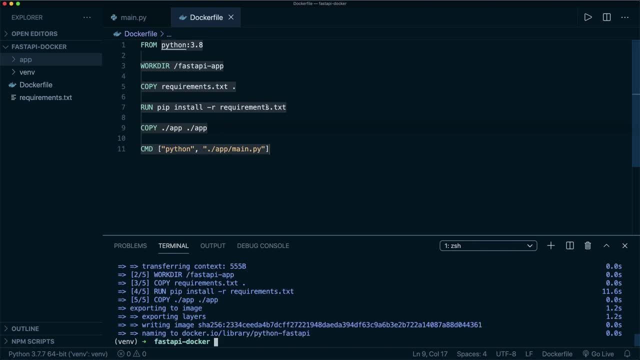 steps. Alright, so this works. So now we have a Docker container with all those dependencies installed. So now we can run this again with the command Docker run, And the name was Python fast API. Alright, so now this is saying that our UV con server is running at localhost 8000.. But now this: 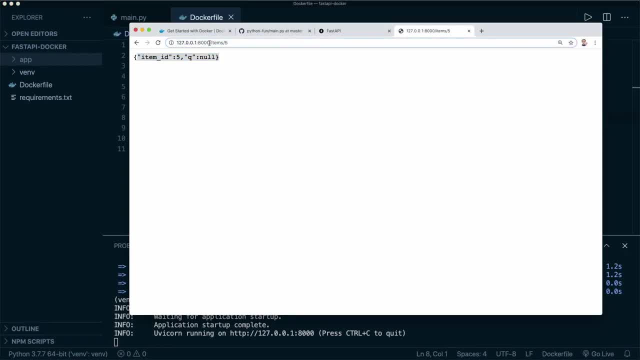 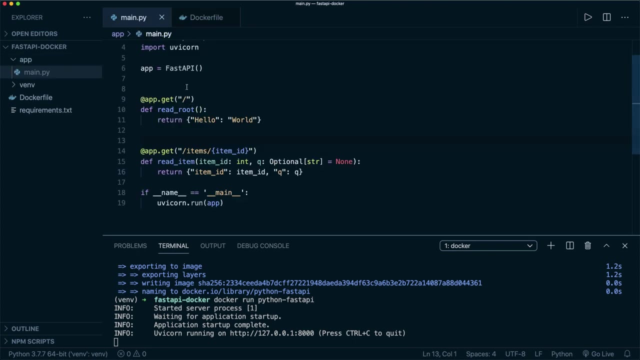 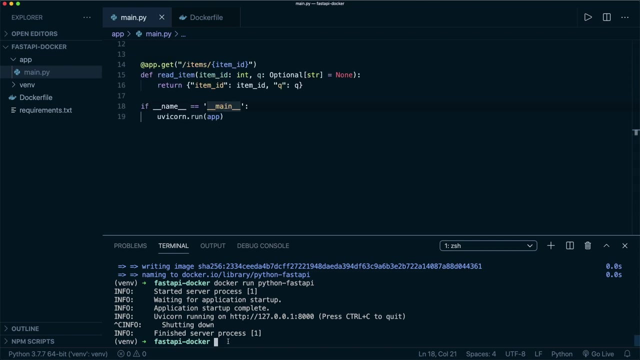 does not work. So if we go to this route again and then hit enter, then we see this site cannot be reached. So for this we have to do some changes. So first of all when we so, let's stop the container again. So first of all what we have to do is when we run our container. 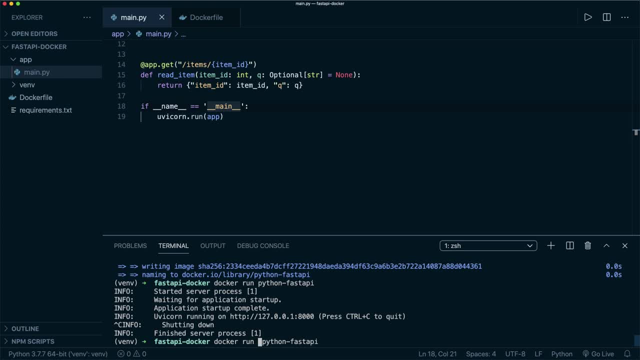 we have to map the port by saying minus p, And then we have to map the port from the outside to the port, From the container, so like this. But before we do this we also have to specify the host and port in our app. So we can do this here in this UV corn run command And here we can put in the 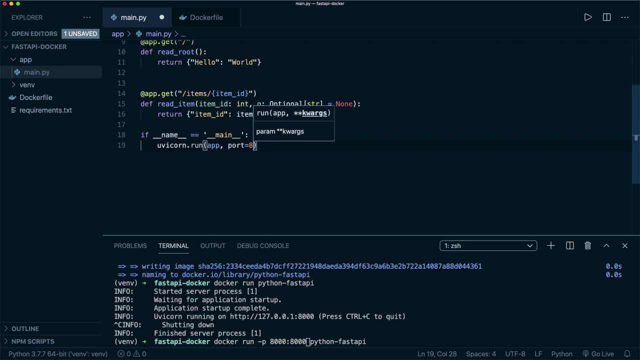 port argument: port equals 8000.. So this is the default anyway. But what is also very important is the host. So we have to say host equals and then here as a string, 0.0.0.0.. This is very important. So this: 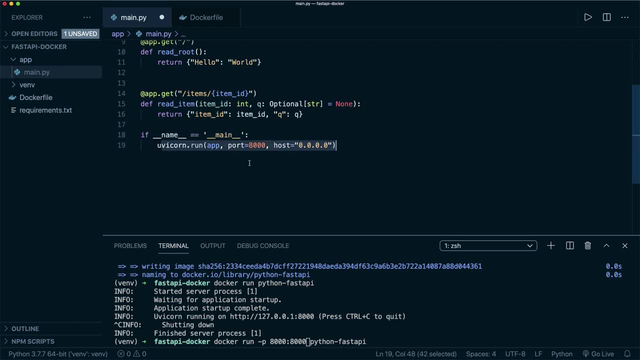 is the same. when we're using this or, for example, when we're using flask, we always have to specify this host address. So now that we have that, what we have to do is again we have to build our image. Now we will add the stare host. So let's say that image here And here. at this stage, 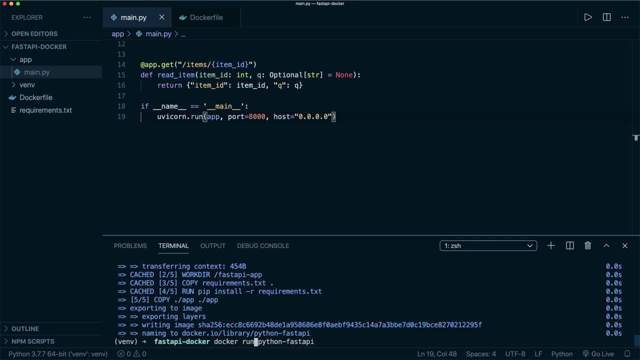 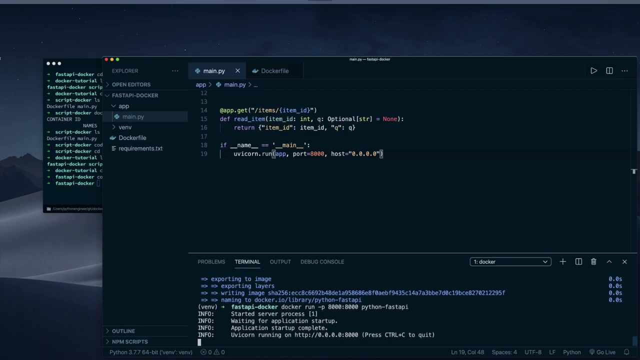 we have to run ourággas attack, So we will build our image in the host brutal amend const And we have to say target console. Hey, now we understand that with this argument. what this means is that we do not need to generate a create key for this image. 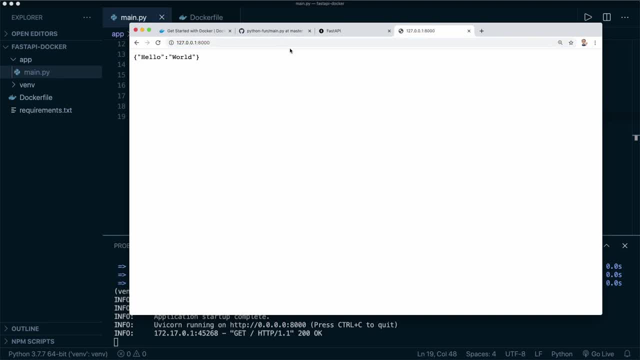 We already have a parent command for our image, And now we can, Vlad, show this now, And this is again the normal example. What we want to do here is to create a system account called target control rug Nous, So when we click on that, we can control this image. And here we have tola. 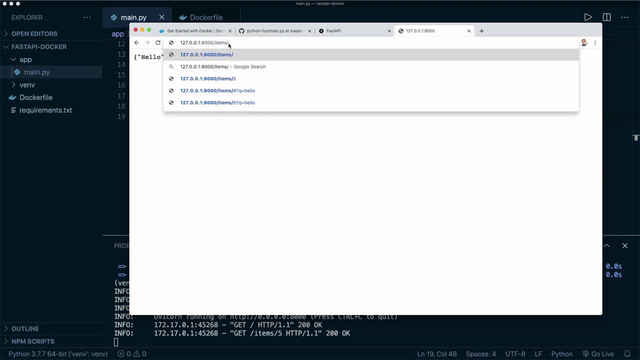 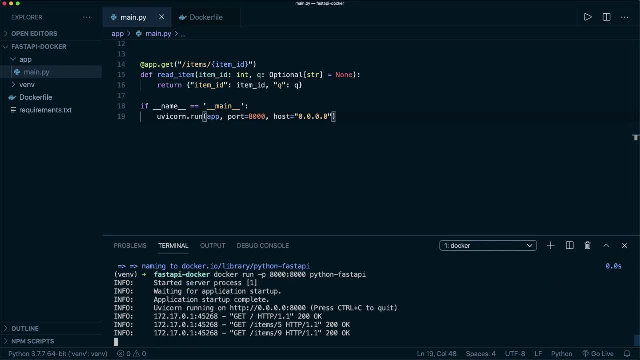 więcej. advanced director console. We chan use our current system to generate the framerate integrations- nonsense- with our also go to items route and then use an item ID. So this is working again And we see here we get the information in this terminal. So yeah, now our web application is running as. 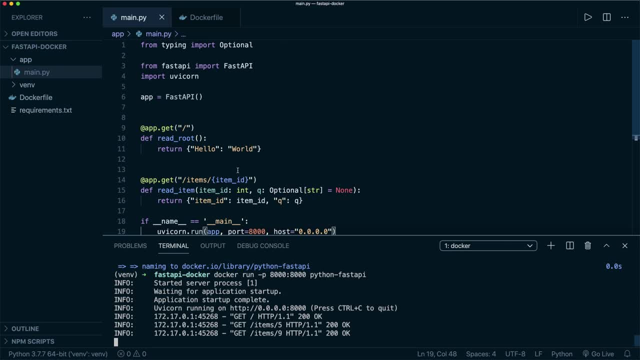 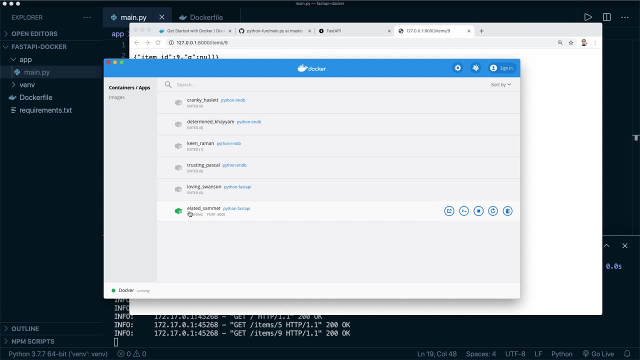 a Docker container. So now, for example, we can go to the Docker dashboard And then here we see that this is the current container. So here we can inspect the locks or delete this or shut it down and restart this. So yeah, the Docker desktop application is very. 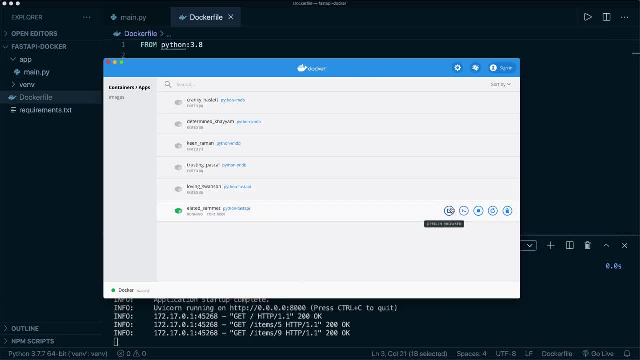 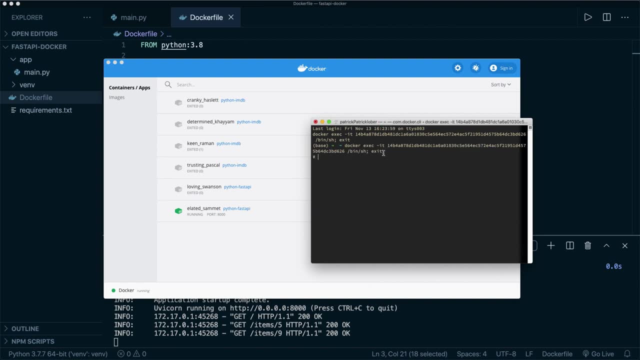 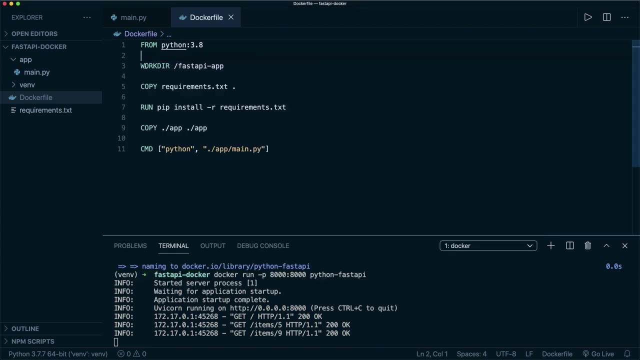 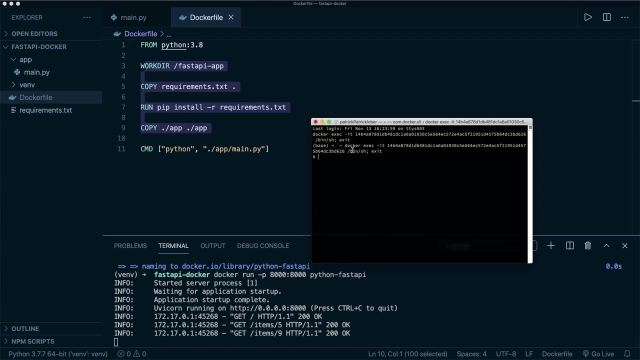 helpful, And what's also very nice is that we can get a terminal inside this Docker container if we click on here. So now we have a terminal, And then I also. I wanted to demonstrate this folder structure again, So this is actually my default terminal. 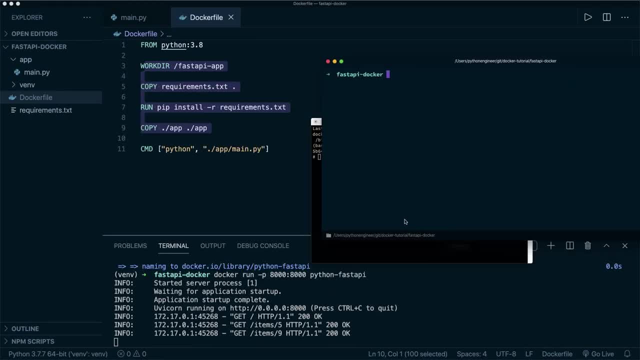 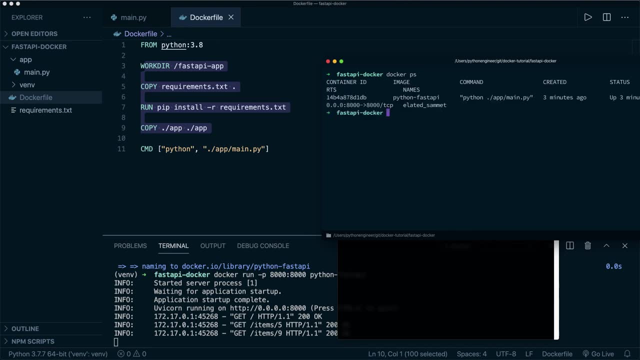 So let me go back to my other terminal And then I want to show you how we can do this with the command. So first of all we can say: Docker PS. this will list all the running containers. So we see that right now this container is running and this is the container.